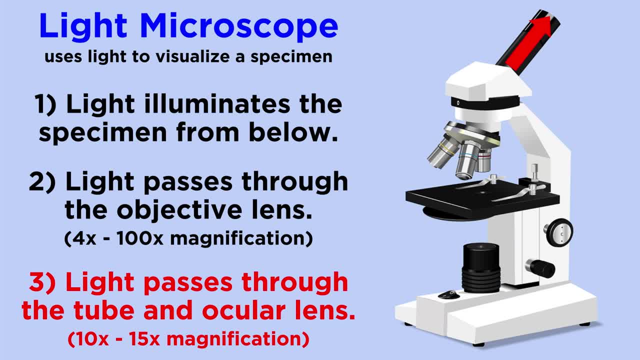 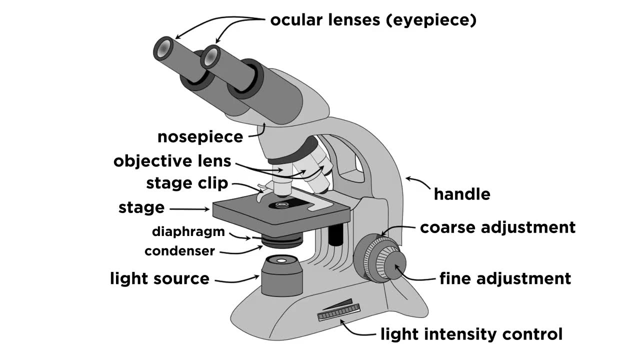 magnifies the image by a factor of 10 or 15, before it finally enters your eye. Some light microscopes can magnify an image up to 1200 times its original size. In order to use a microscope properly, one must know the names of all its components. 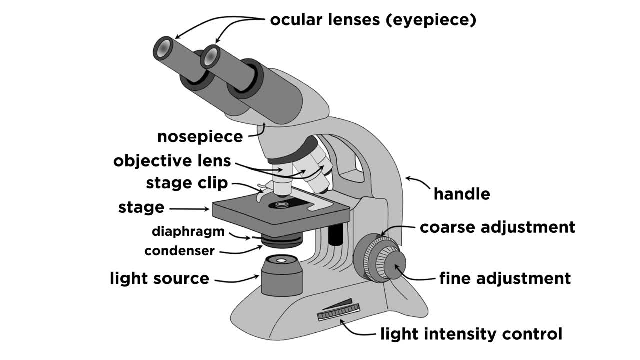 as well as their functions. So let's take a look at a typical light microscope. Any light microscope has a stage that the specimen sits on and stage clips to hold the specimen in place, which is usually nestled between a slide and a coverslip Attached to the stage. 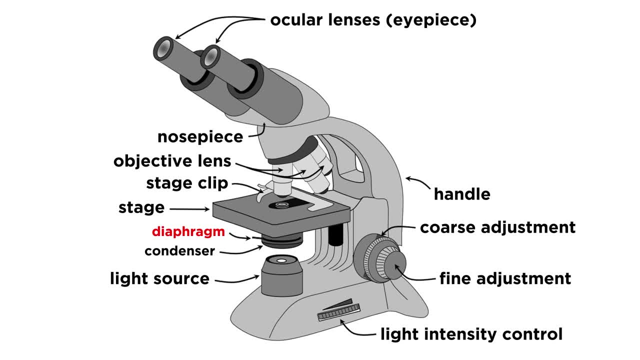 is the diaphragm, which controls the contrast of the image by controlling the amount of light from the light source. On the sides of the stage are the slide adjustment knobs which are used to move the specimen so that what you want to see is in your field of view. Above the stage are the objectives. 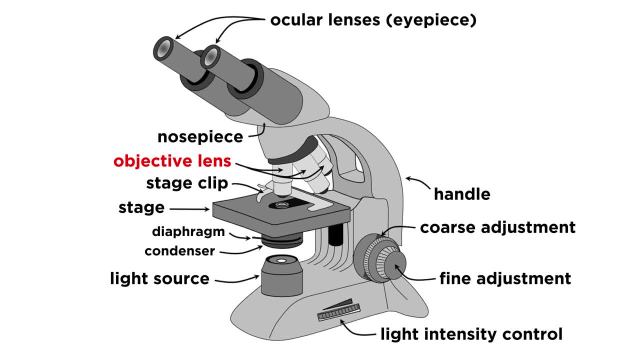 that are held by the nosepiece, which can be rotated so that different objective magnifications may be employed to view the specimen. The tube of the microscope connects the nosepiece to the eyepiece, which further magnifies the image, and is then moved to the eyepiece. 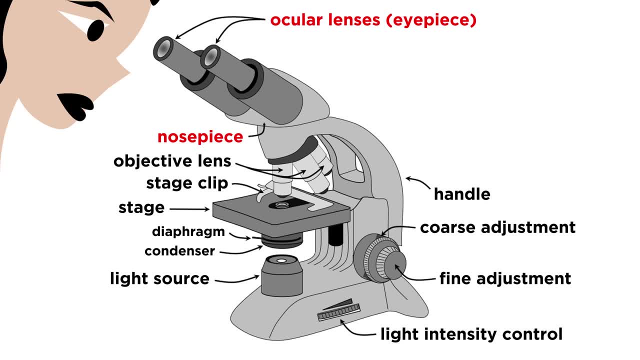 This is the part one looks through to view the specimen. There are also focus knobs on the side of the microscope, the larger one being the coarse focus knob, used for larger changes in focus, and the smaller one being the fine focus knob used for smaller adjustments in focus. To put these parts to use, one can start by plugging. 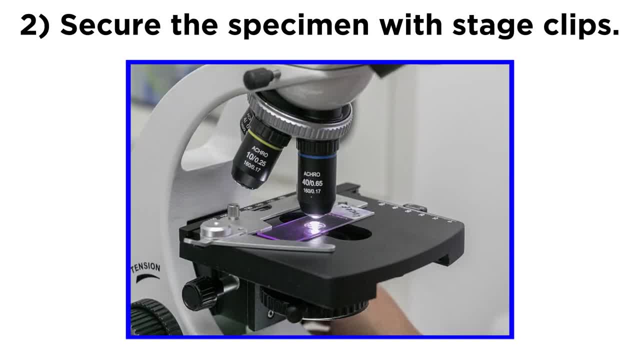 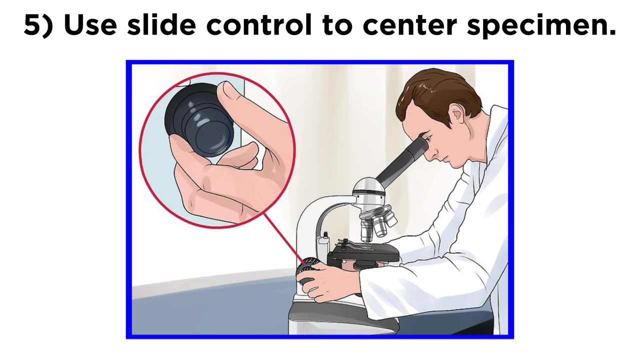 the light microscope in and turning on the light source. Then secure the specimen on the stage using the stage clips. Before rotating the nosepiece so that the smallest objective is in place over the specimen. First use the coarse focus knob to clear up the image. then use the slide control knobs. 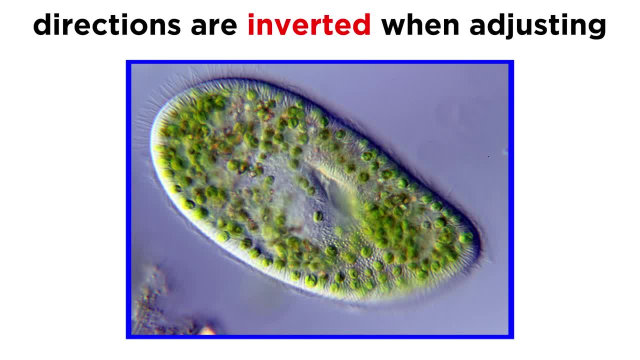 to center the specimen in your field of view. A tip for this is that the image in the microscope is inverted, so when you move the slide to the right, it will move to the left in your field of view, and vice versa. Next, use the fine adjustment knob to refine the image. 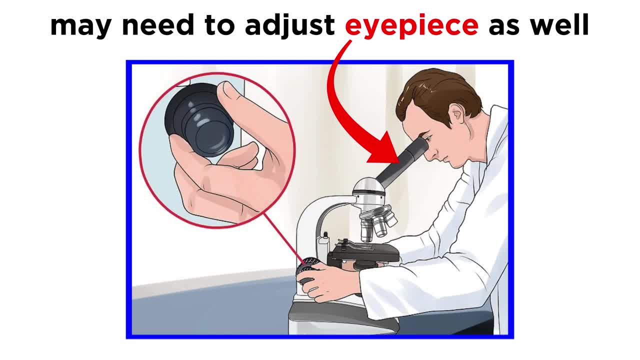 This can also involve adjusting the eyepiece or eyepieces to further focus the image of the specimen. A tip for adjusting eyepieces is that if there are two eyepieces, the focus for either eye might be different, given that your eyes are not identical. Additionally, the focus setup. 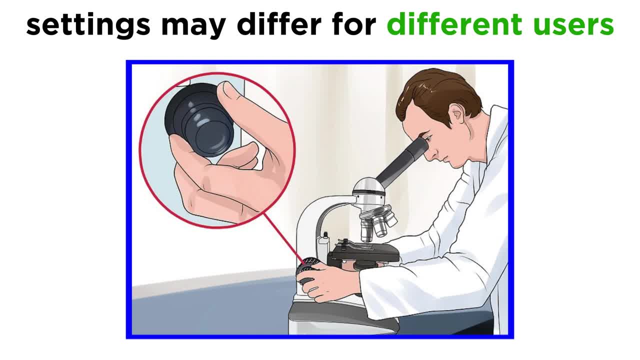 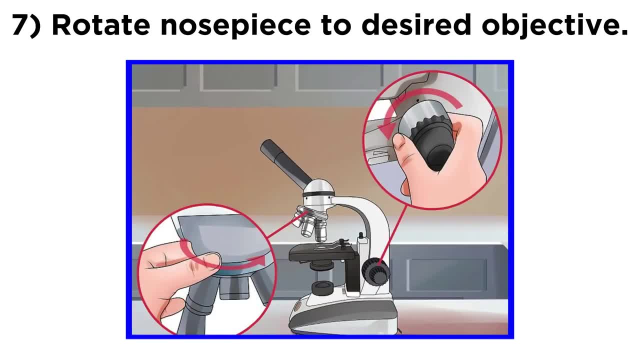 differs slightly between individuals with different prescriptions. Each person may have to readjust the focus when using the microscope. After the focus is set, rotate the nose piece objective appropriate for your purposes. Usually, between switching objects, it is necessary to use the fine focus knob to clear up the image, but avoid using the coarse focus. Make sure to note. 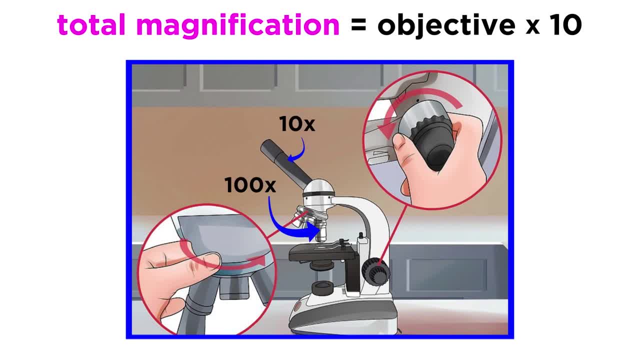 what objective you are on when you make observations. Also, note that the total magnification will be 10 times the objective, as most eyepieces magnify the image further by a power of 10.. It's important that when using the 100 times objective, it is set up for oil immersion to. 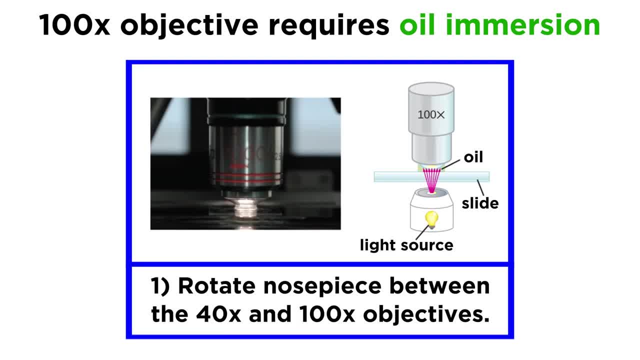 improve the resolution of the image. To do this, rotate the nosepiece so that the specimen is between the 40 and 100 times objectives and add a drop of oil on top of the coverslip which sits over the specimen. Then rotate the nosepiece so that the 100 times objective is submerged. 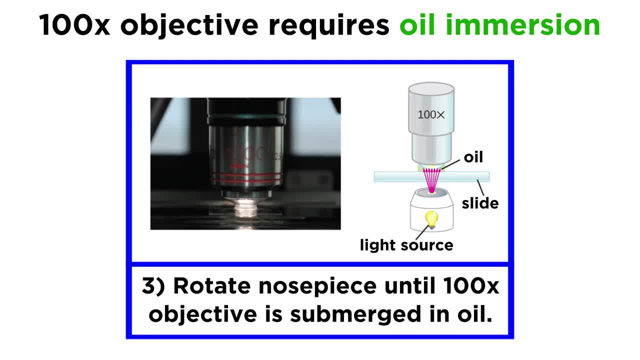 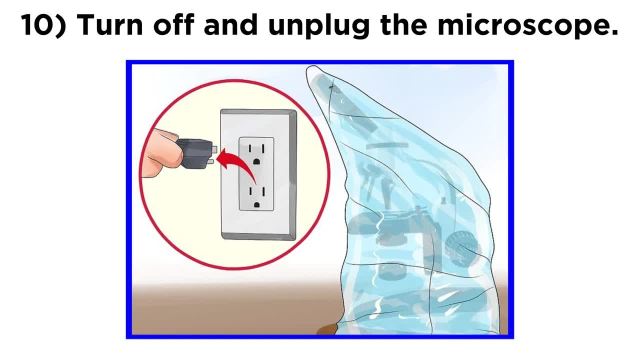 in the oil and over the specimen without scraping the lens. Finally, after making all of your observations with the light microscope, you will need to turn off the light source, unplug the microscope, dispose or save the specimen properly, use lens paper to. 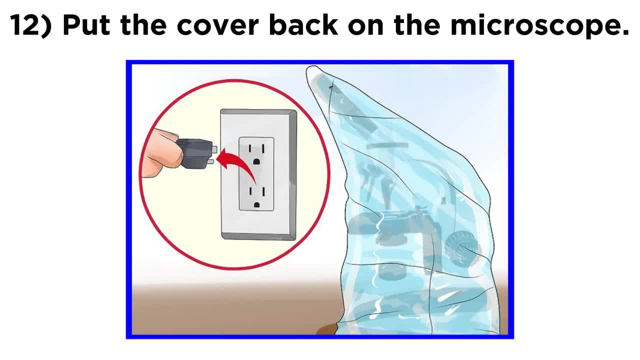 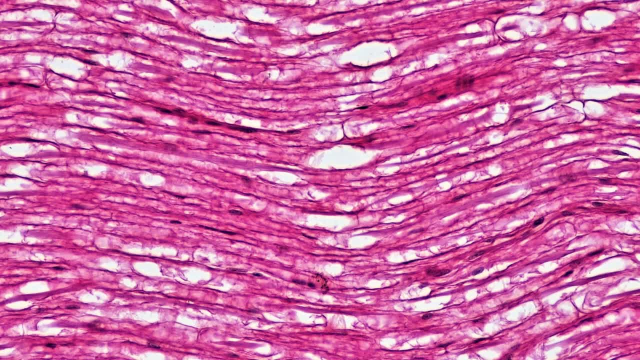 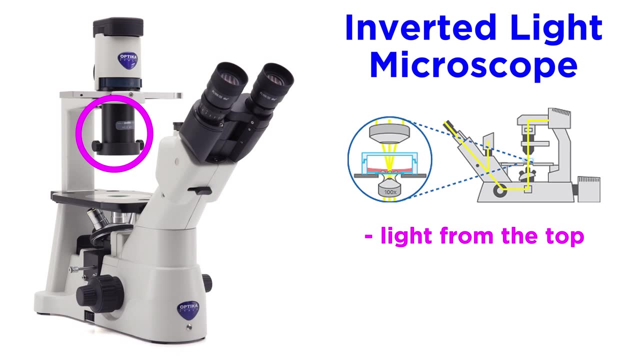 wipe off any oil on the lenses and replace the microscope cover. Light microscopes are commonly used to study bacteria, slices of tissue, liquid samples and some mitochondria. Inverted light microscopes, which have the light source coming from the top and the objective. 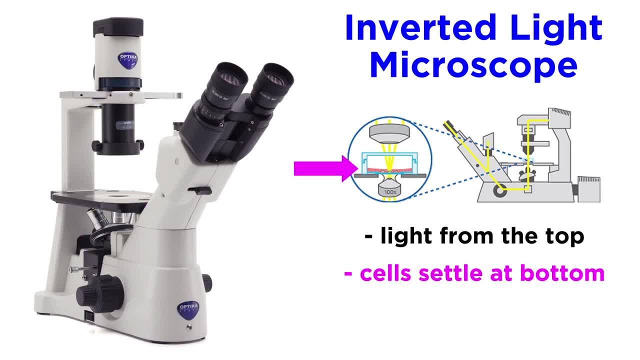 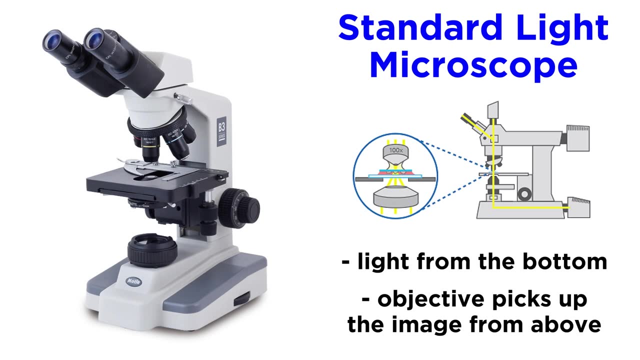 under the stage are often used to study tissue cultures like cells covered by liquid media. as cells settle to the bottom of the flask, where the objective can pick up the image, This is in contrast with a standard light microscope with the light source below and.